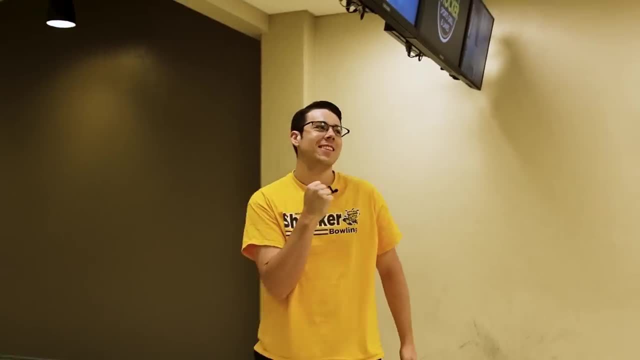 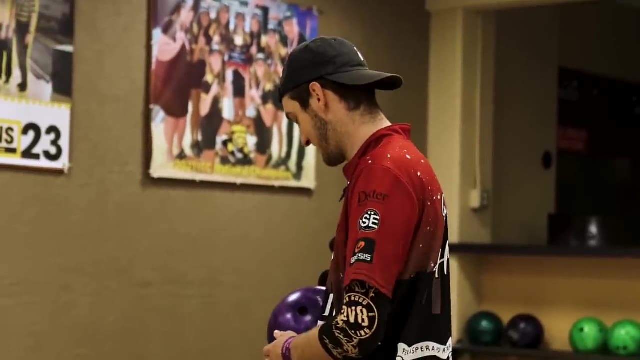 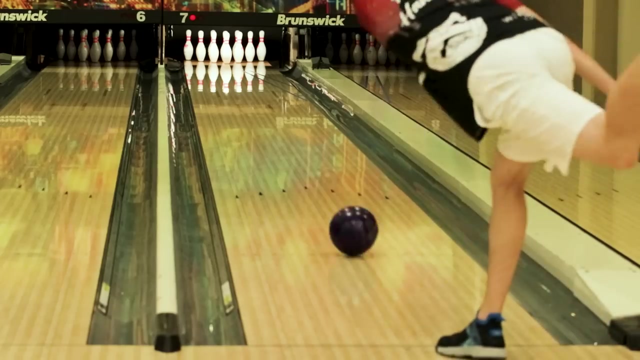 Go Brooklyn. That's what we needed. It's okay, I'll strike here. Come on. Matt just had to hype him up by saying he was the six pound ball champion, Channeled it right back in Eight pound strike. Now we got the nine pounder Purple ball. Yeah, they do. Oh, That's devastating Tough break. 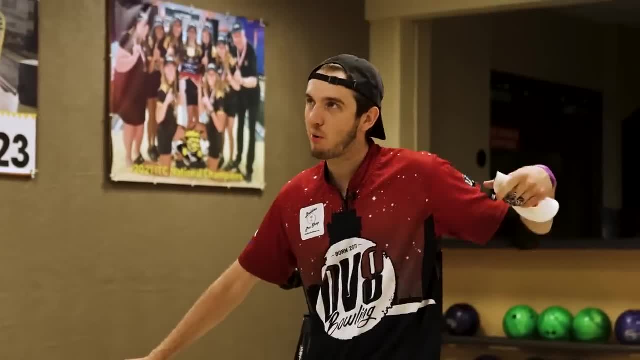 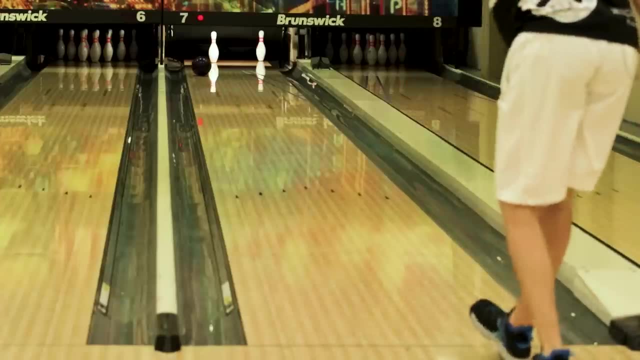 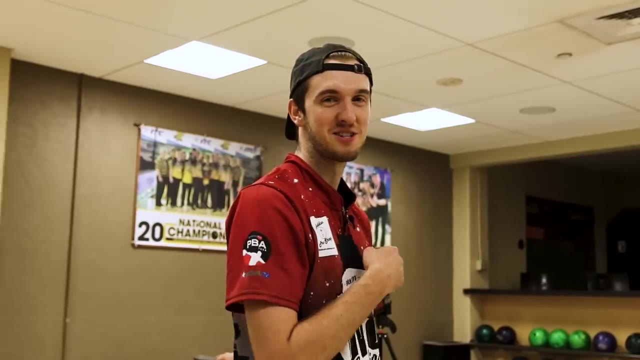 I bet I could bounce this. Send the ball across the deck. Yeah, I keep pulling it down from the top. It's just not good. It's like the ball is like nine pounds. Oh, Tough break. That one hurts in here. Sometimes you just make good shots and it doesn't pay off. 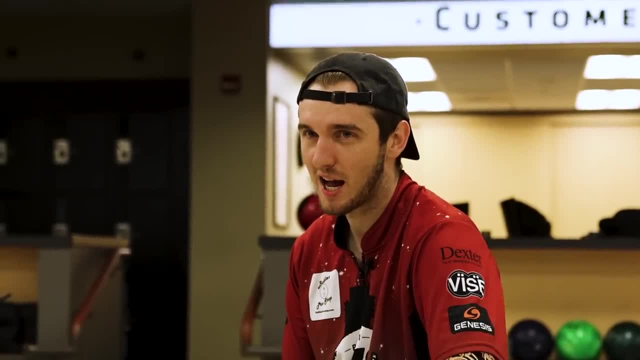 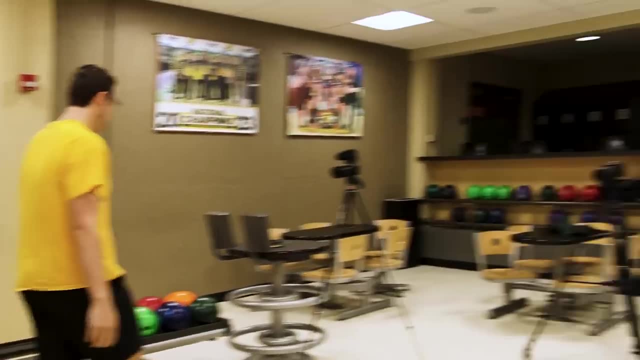 Yeah, the Brooklyn 210.. And then I laced the spare shot Brooklyn. Oh no, Oh, Hooked too much. That is a tough spare, if I've ever seen it. You have to hit the right side and you can't hit it too thin or it's going to bounce off. 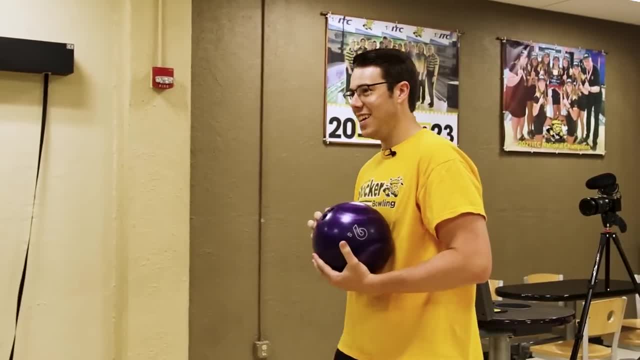 Right now, I wouldn't want to be you. Do you throw a back up ball at it? Oh I might. I'd think about it, that's for sure. No, we'll get spicy with it. I give it some thought. The left side is always easier. 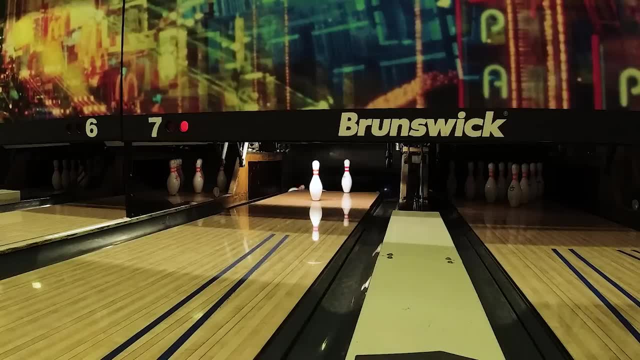 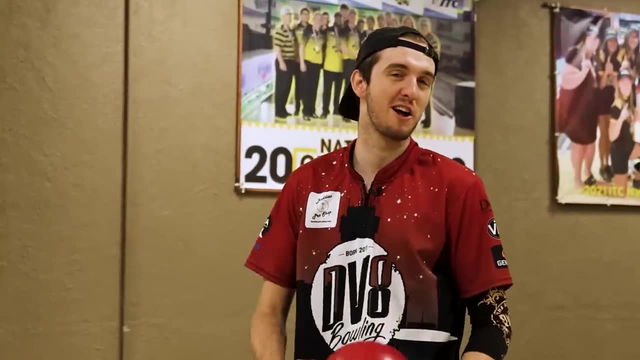 Oh, no, No, no, no, I tugged it and threw a back up ball. You are the only one to strike, but you know, as they say, spares for dough, Strike for show. This video today is brought to you by our sponsor, Element. Today we're getting our electrolytes in Super quick. I'm going to rank the eight flavors that come in this Element sample pack, So my bottom two are my least favorite are the raw unflavored and the chocolate salt. What's your favorite part of Element? My favorite part of Element is that it's an easy way to get my electrolytes on the road when I'm doing all this travel. My next two are lemon, habanero and the citrus salt. My next two are going to be orange salt. And mango chili. It's been super hot in Wichita lately when I've been working out with Andy. This is one of the easiest ways to replace all of that sodium, Which there is a thousand milligrams of sodium per pack. And then my top two, my two favorites: the raspberry salt and the watermelon salt. 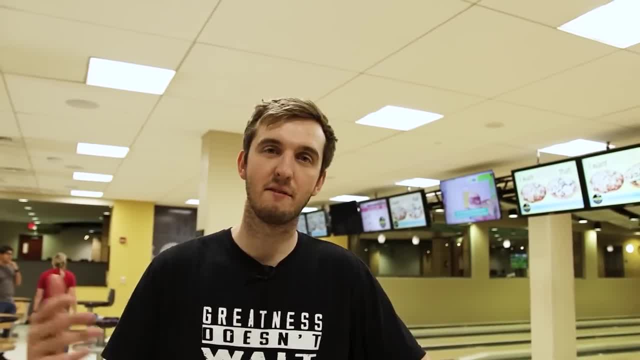 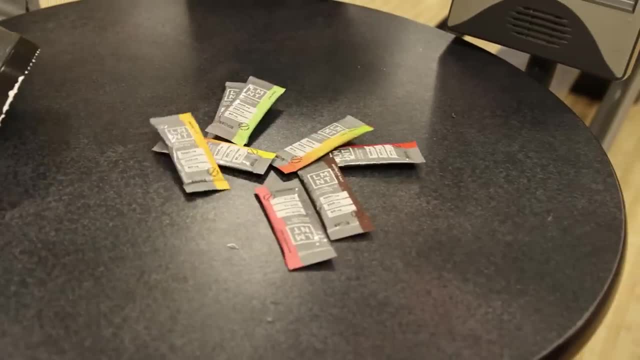 Both of these flavors, I just think, are absolutely delicious. These are the ones that I drink probably every other day whenever I go and work out. Right now, Element is offering my viewers a free sample pack with any order. That's eight single serving packs free with any Element order. 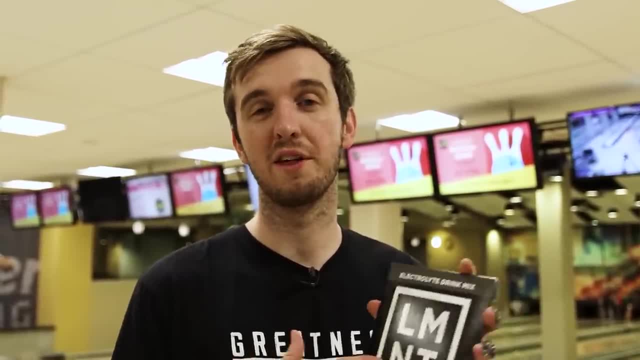 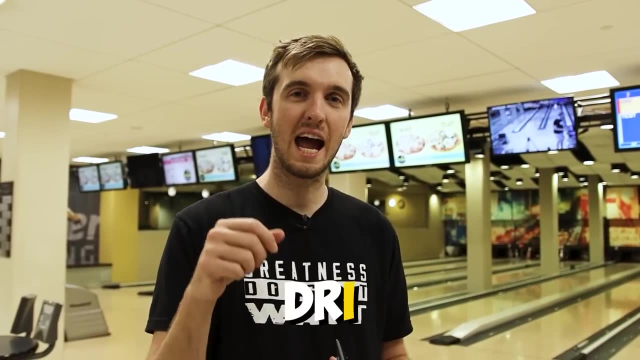 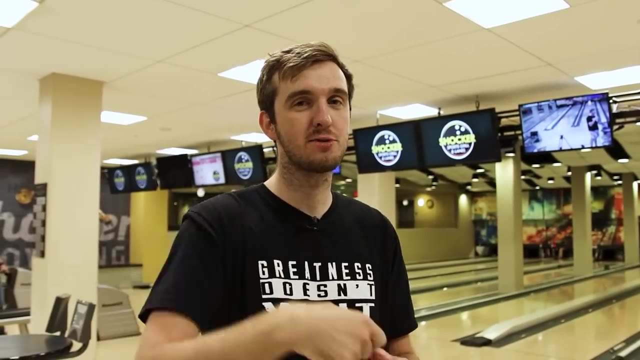 Great way to try all eight flavors, or share Element with a salty friend. You can get yours at drinkelementcom slash house. That's going to be d-r-i-n-k-l-m-n-t dot com slash house, And for those of you who missed it, the link is also down below in the description. 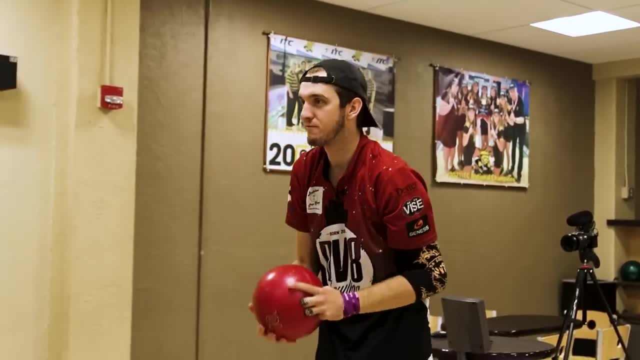 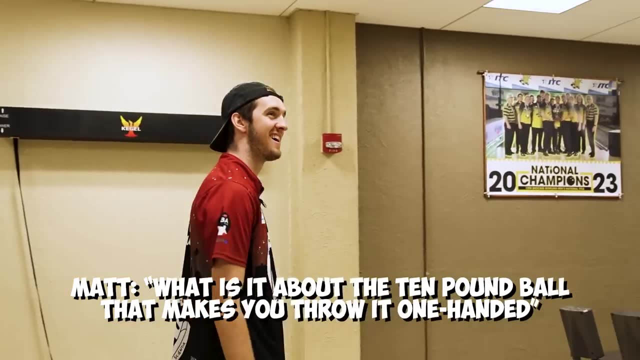 And now let's get back to bowling. Ten pound ball- fireball. I'm about to skimp out until you have to throw it. I'm about to skimp out until you have to throw it. I'm about to skimp out until you have to throw it. 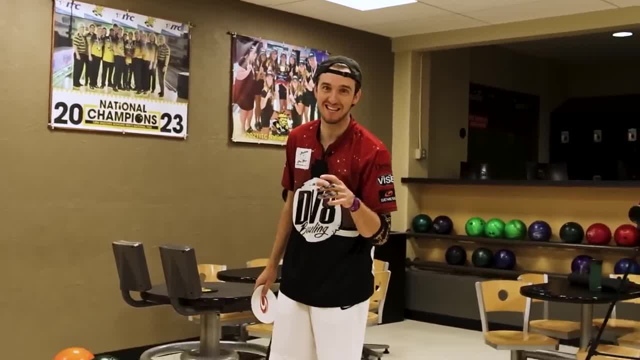 I'm about to skimp out. I'm about to skimp out until you have to throw it. It just fits my hand perfectly. I always hit the pocket. That's why, And my wrist always feels like it's going to explode when I'm done. 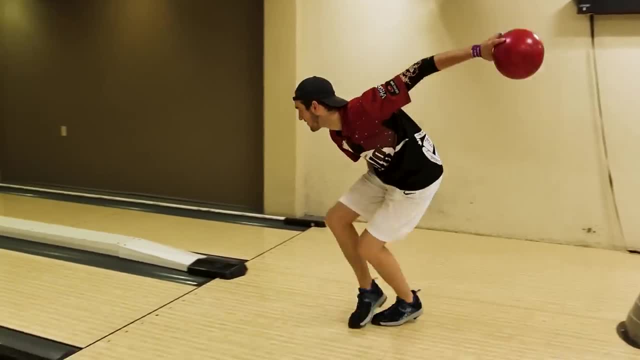 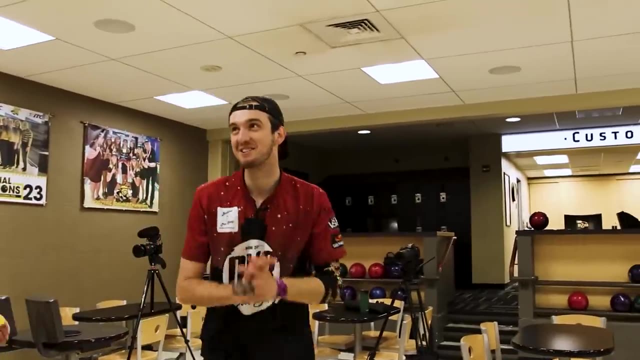 I got to make a spare And it's not going to be one-handed. Yeah, it is. I love it. You like that? I really, I really tried to get. I tried to get low on that one. Let me know if I can fit my thumb in this one. 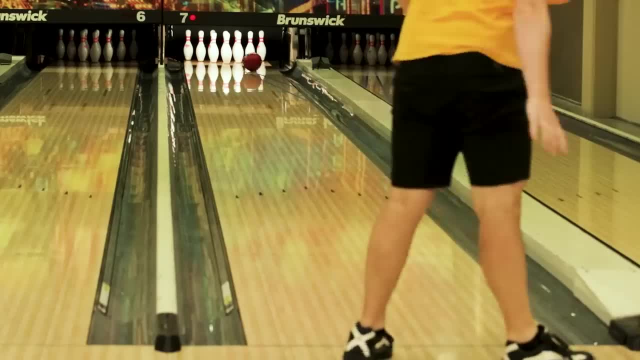 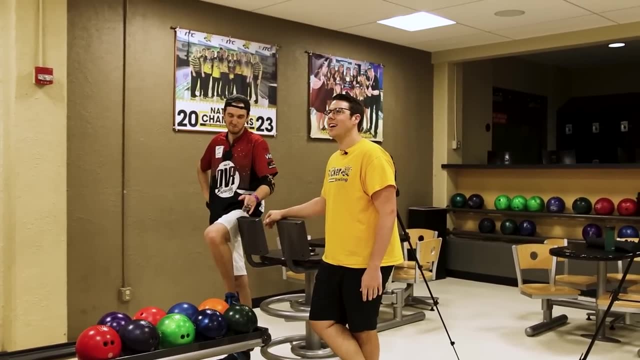 This might not come out. Oh, What the heck was that? I was kind of scared it was going to get stuck on the thumb. The good news is: the higher up in weight we go, the bigger the finger holes get. Yeah, So I know it won't stick. 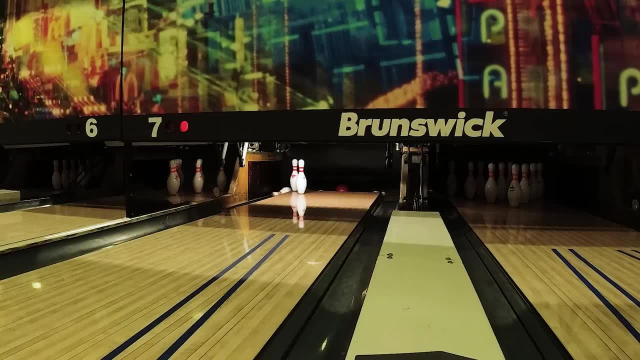 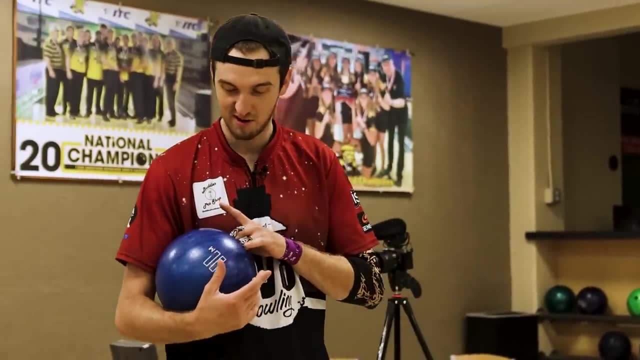 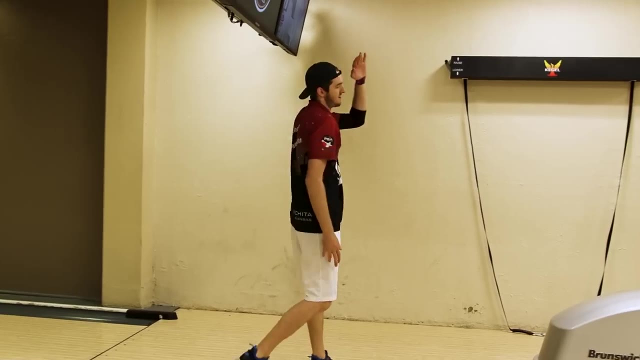 Push, Oh, Am I going to get 100? this game, Plastic ball champion is going down. You might want to find another 11 pound ball. I'm just letting you know. These finger holes are so long, Oh my God, He's shaping them. 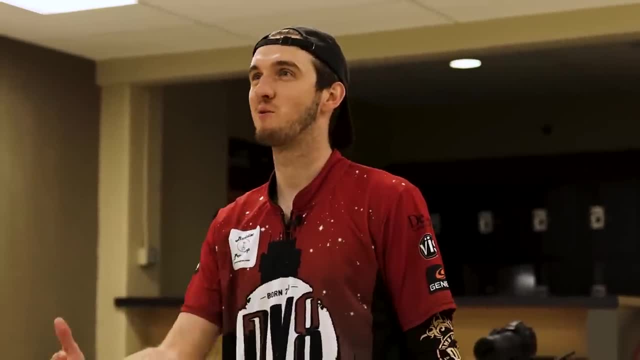 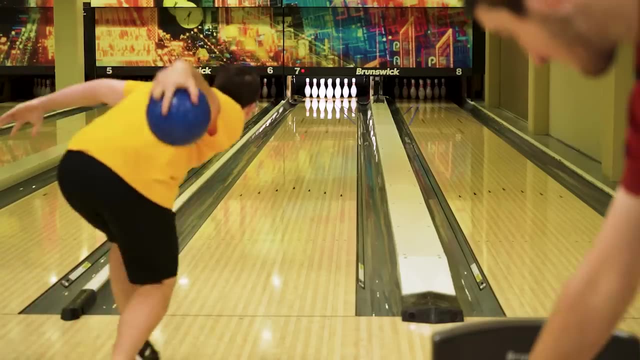 We talked about tryouts at Wichita State. This is my tryout, line 23, all the way out to like 13.. As long as I get a spare, I think I'll be okay. Oh, that's pretty good. King of the Brooklyn. 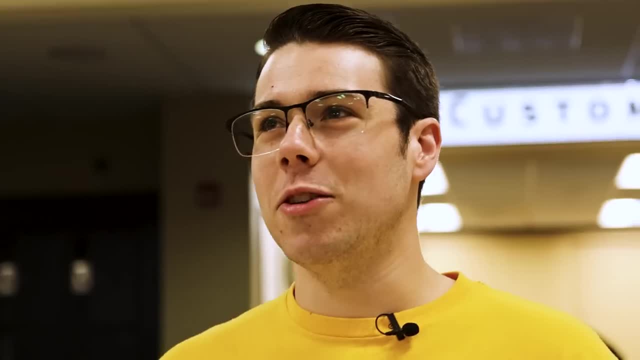 Let's go. So is this how Madison feels? every video: You know: when you hit the left side, you're going to strike. That's just what happens, Right Packy. It's a guaranteed strike on the left side of the lane. 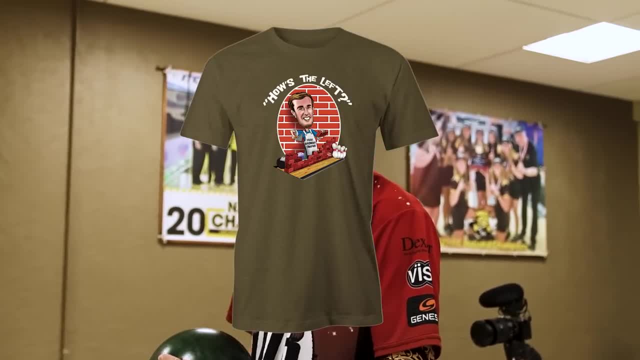 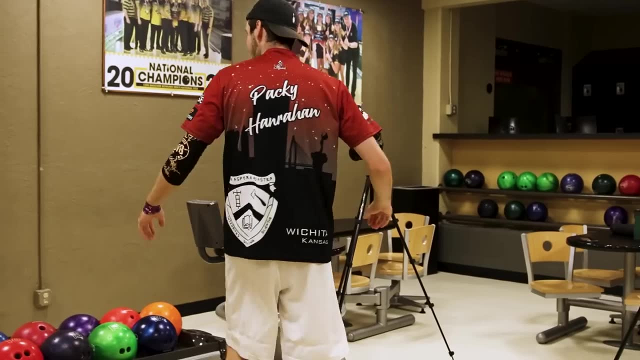 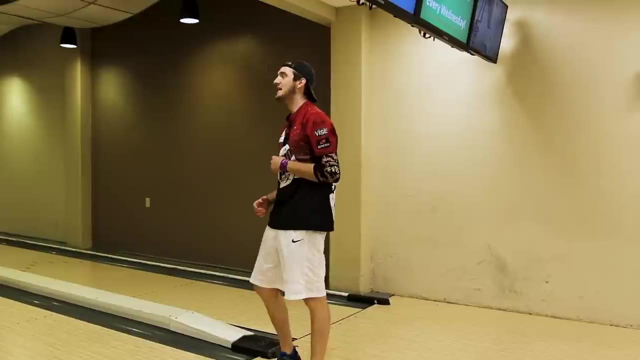 Because the left side is always walled. Insert clip of merch Buy if you want. All right, Oh, that's hooking, I can take that And that's why you play that line. Oh Yeah, baby Golly. 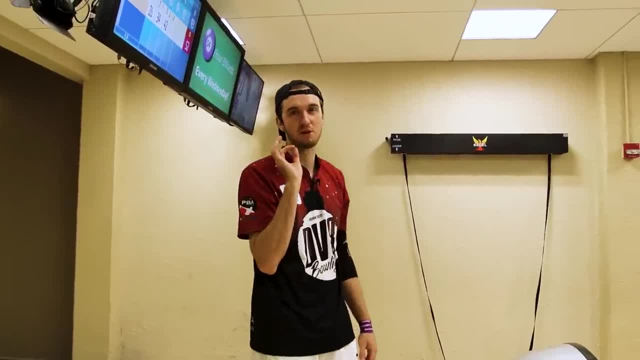 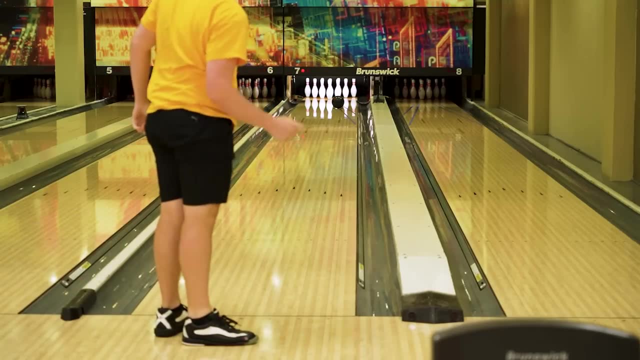 I literally said if you just throw the same shot, you just threw on your strike shot, but just throw it better. I did. It just hooks a little bit. That's way better than mine And that's why you go Brooklyn. Bad thing is I have to shoot the spare. 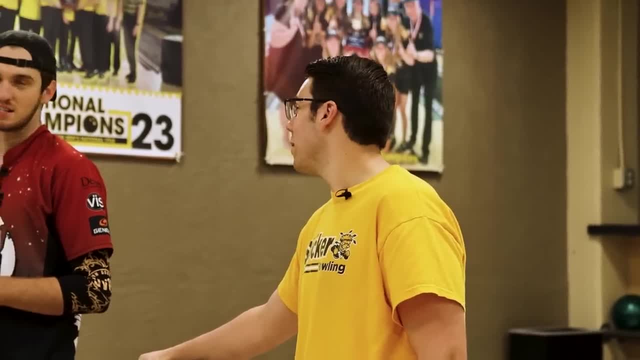 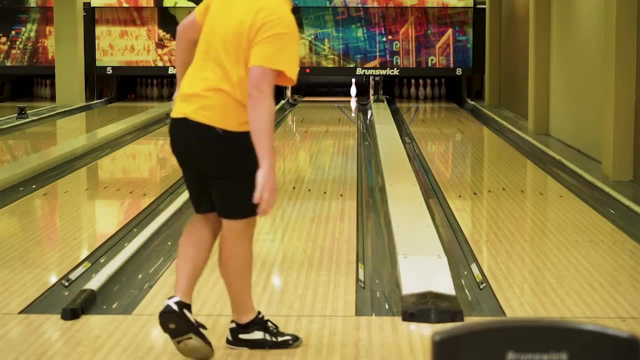 Not feeling so confident on the 10 pound. 10? Not without the thumb in it. Can I fit a quarter of my thumb in the ball to make the spare? Hey, that ball hooks, I'm telling you. I'm not saying that that was a big time spare. 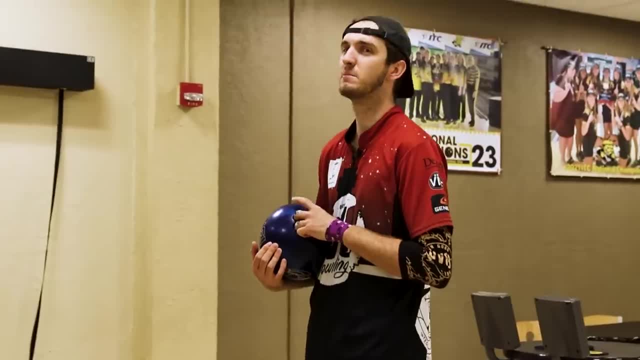 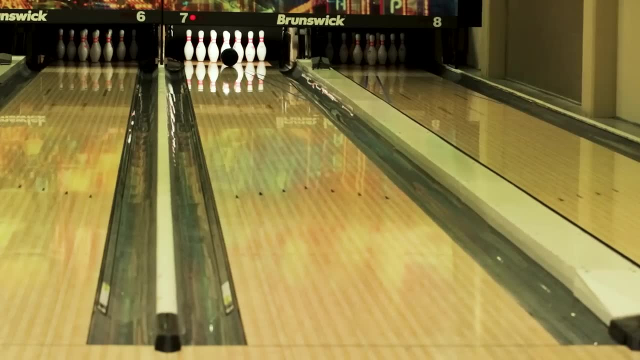 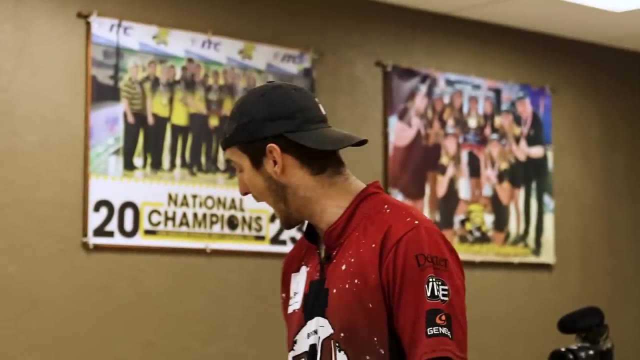 but that was a big time spare man, That was a big spare that I flagged. I could beat you one handed Probably. Watch and learn. Oh, it's flat For some reason. I really thought that was gonna strike, Golly. 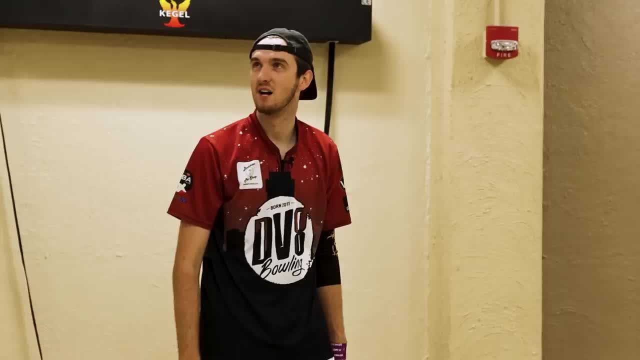 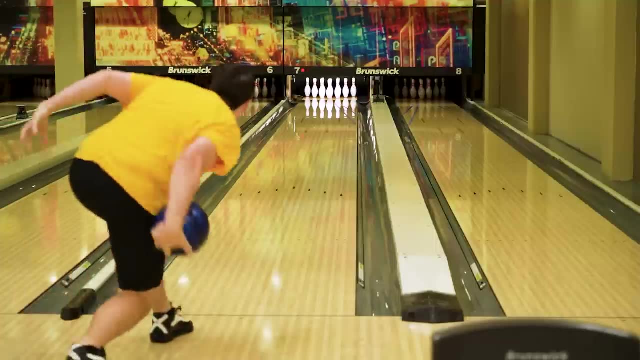 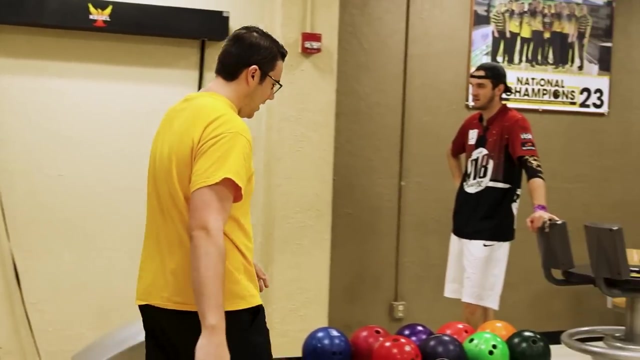 Oh, It's all right, I still got this match locked up. He says that We're getting into the heavyweights, though It hooked, Don't fall forward. I needed that to fall Like, even if you do win. 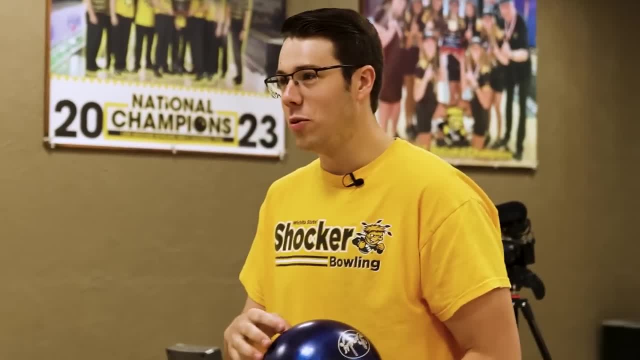 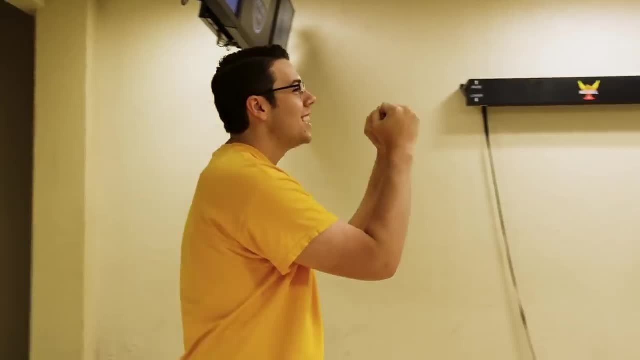 you're gonna get paid very little amount of money with these scores And then we get like $12.. Uh-oh, Yes, Wow, Let's go. Wow, The 13 pounder has always been a favorite of mine. 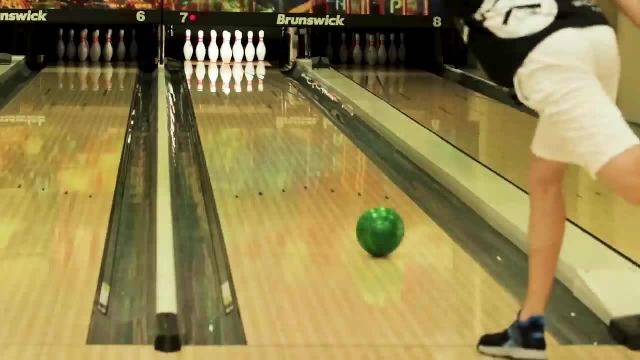 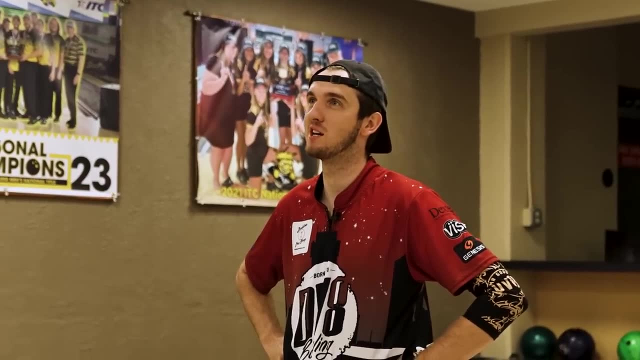 Just like it really fits my hand. well, Stand up and fight. To be honest, I don't know why I'm throwing these shots one handed, but it seems like they're doing better than when I throw them two handed. Oh my God. 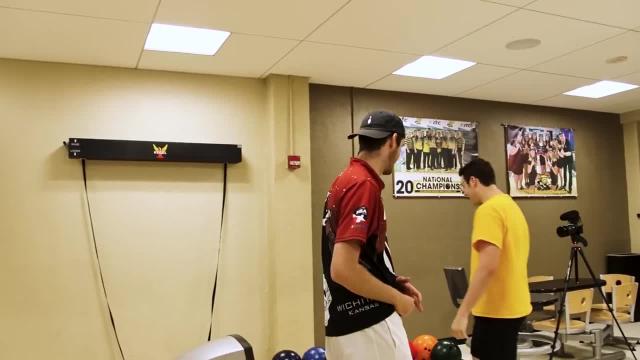 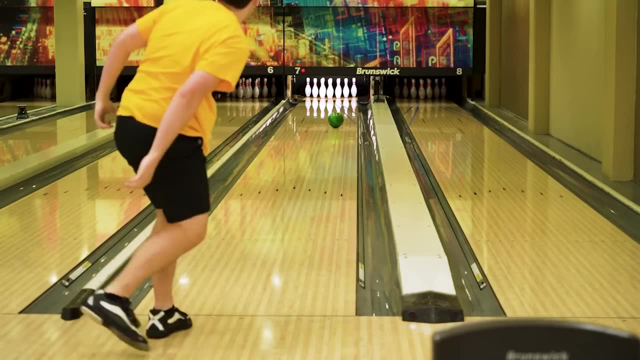 My finger legitimately slipped out of the bowl. Uh-oh, I should've stuck to throwing it one handed. That's the easier way to bowl. You heard me Bang. All right, I'm in trouble. Split the eight- nine. 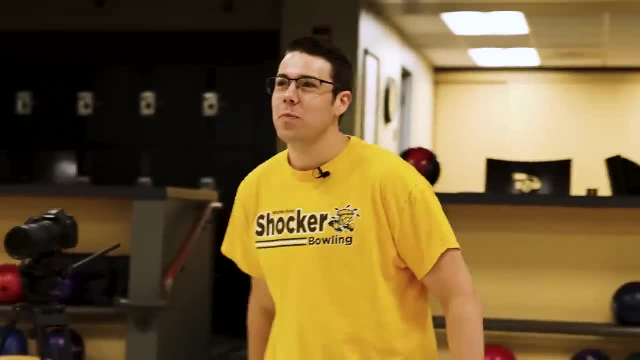 Come on, I'm officially down. Let's go. I'm not officially down, but I'm unofficially down. All it took was two frames, two marks. We're there. We're there now. Ninth frame: 15 pounds. 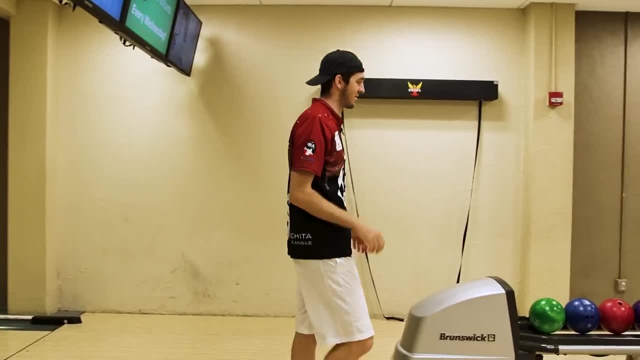 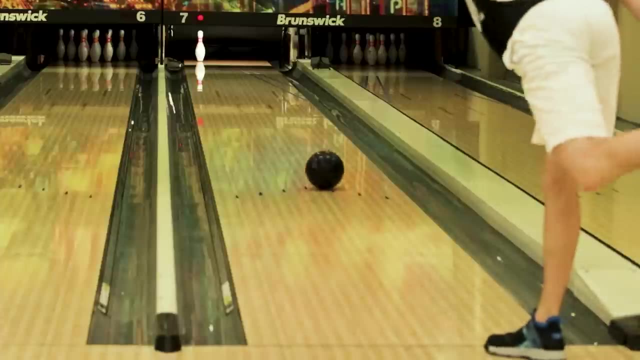 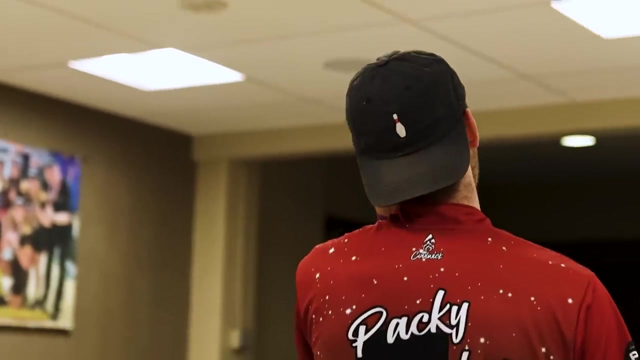 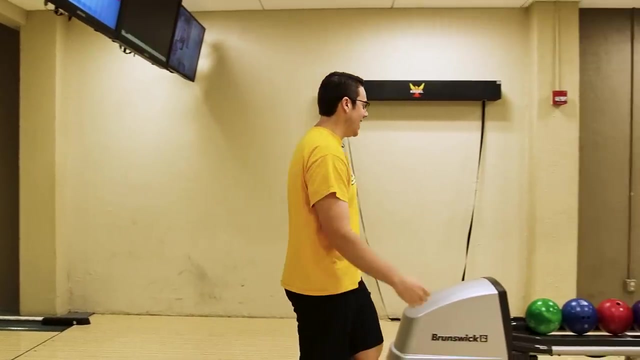 Brooklyn: The heavier balls don't hook. Single pin redemption. I'm 0 for my last two. The first ball has not been the issue, It's the second ball. Oh, It hooked again. Thank God that it stood up. God, I thought that was a double. 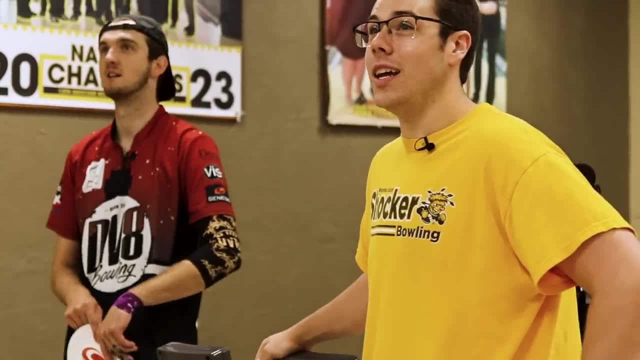 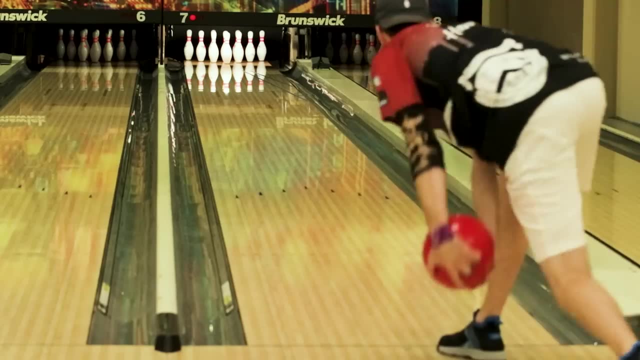 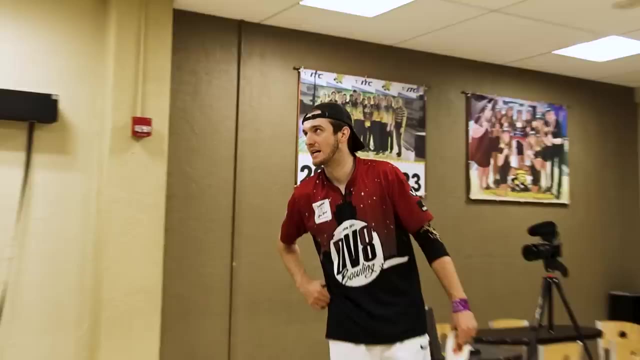 Hopefully I can make this single pin one handed with my thumb in it. Miss it. All right, I need a big 10th here. I can make this spare, but I really needed like a strike, Like I needed it. I got Brandon on the count factor. 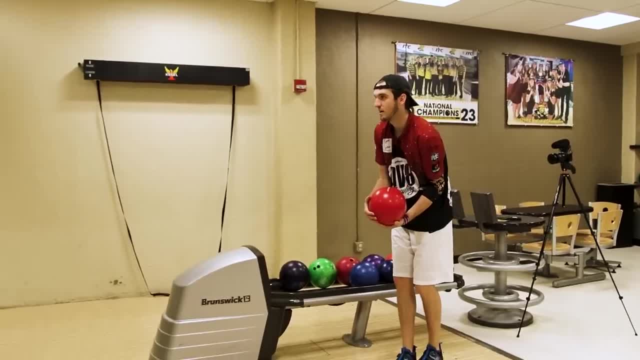 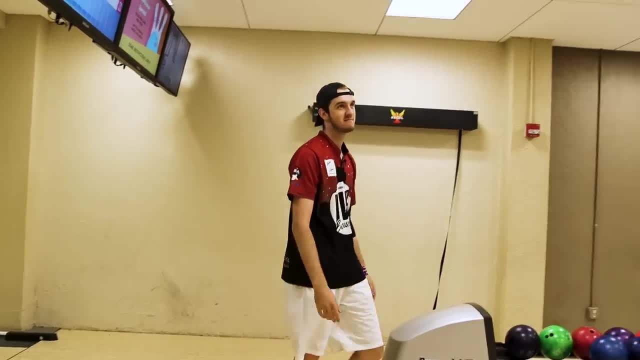 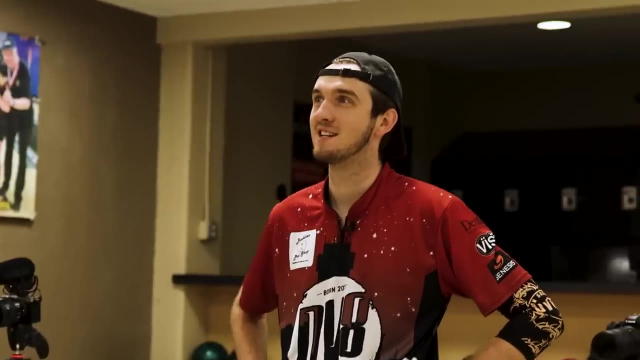 so spare strike here forces him to mark Key word: spare. Something about the middle of the lane. I'm telling you The middle lane is on fire. They're hooking. I'm 0 for my last five frames. I felt good. then I shot 120.. 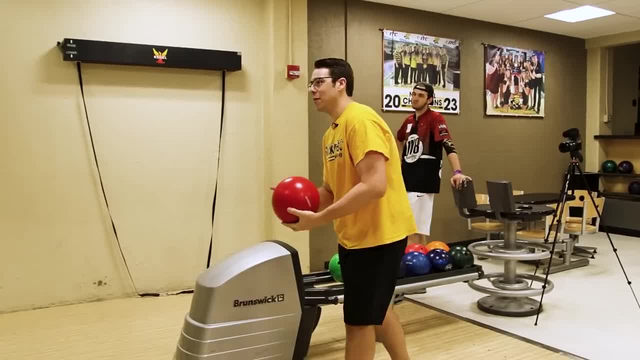 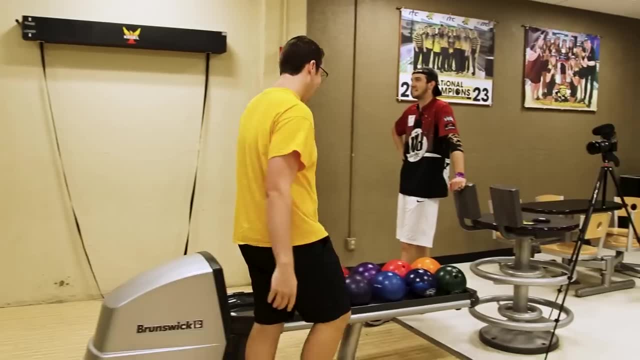 Crumbled this game: Absolute collapse. My fingers are just feeling like they have arthritis the further I go in. Oh no, Oh, my God, He's gonna make this thing close. He needs a pin. I didn't know. I grabbed the 2X 16 pounder. 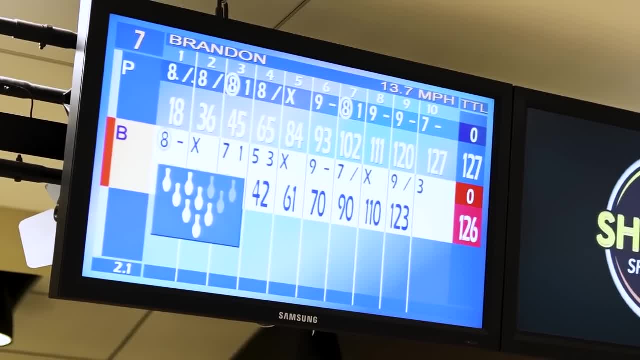 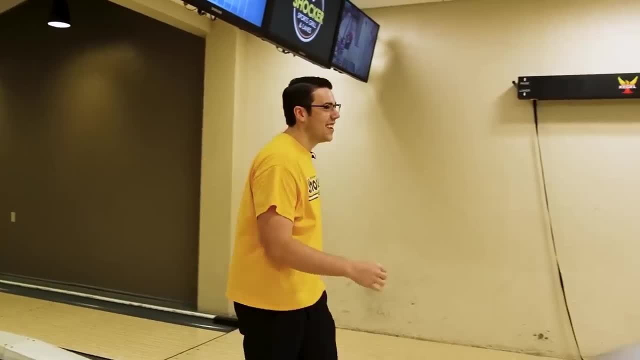 Yeah, sorry about that. I think that's all we got here, So I need to keep it on the lane. Well, you can keep it on the lane and still get zero, Just saying: Oh you lucky, Yeah, baby. 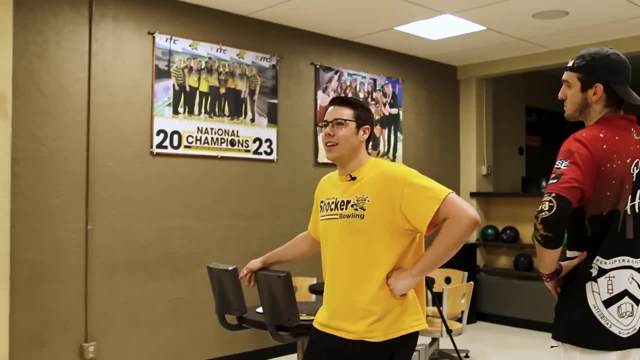 And he got a spare. Increase that average, try and get that money. Hypothetically speaking, we go into a ninth tenth frame roll-up. What kind of weights are we using? 16 on the first, six on the second. 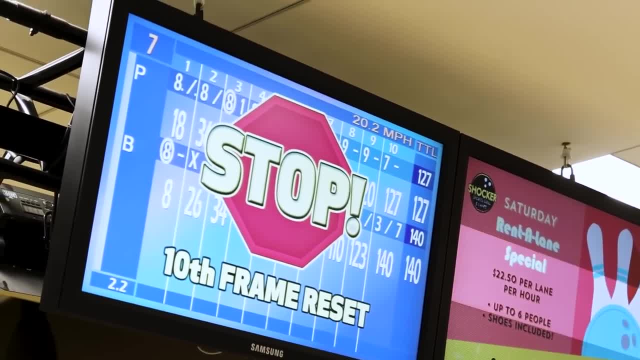 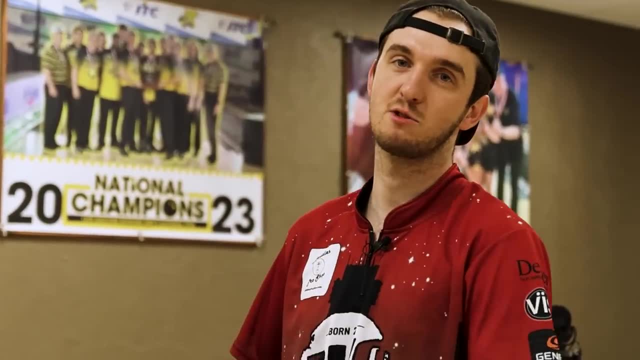 Yeah, we can do that. yeah, All right. Game one winner. due to an absolute collapse from me, I need to win the next game. Now we're going 16 pounds back down to six for game two and I need to win. 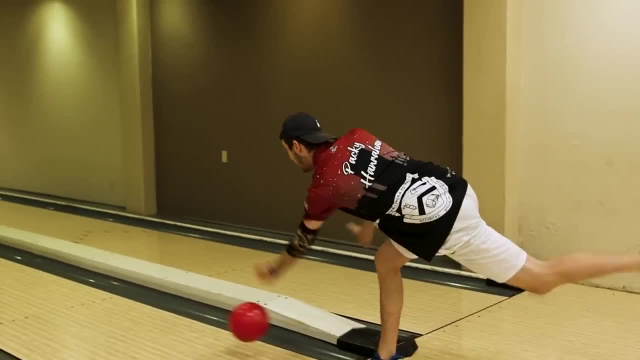 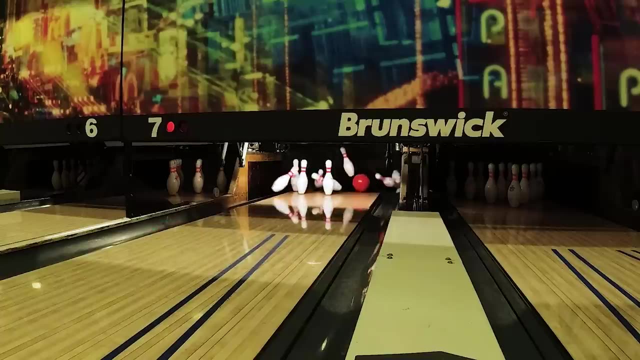 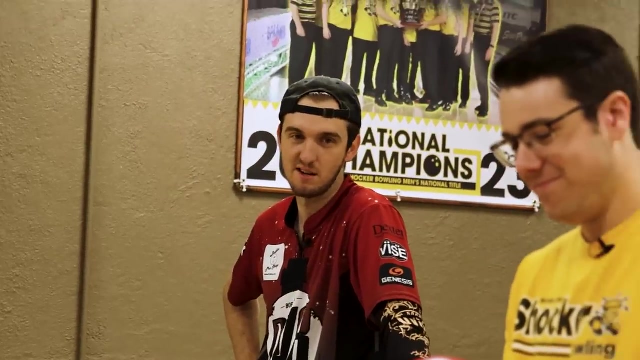 Otherwise I'll be paying the man. Oh, Ah, Oh, Oh Oh. Striking is the easiest way to make your spares. Amen, I physically cannot stop missing, right, I'm tracking over all the finger holes. yes. 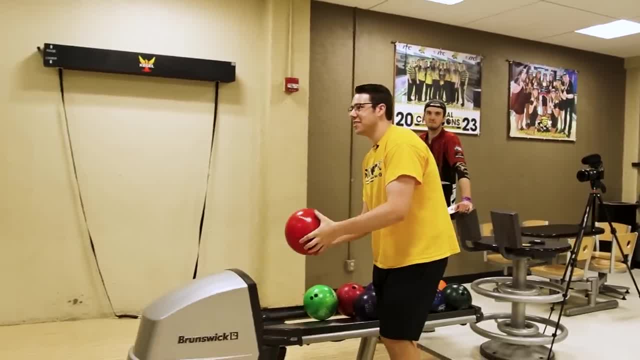 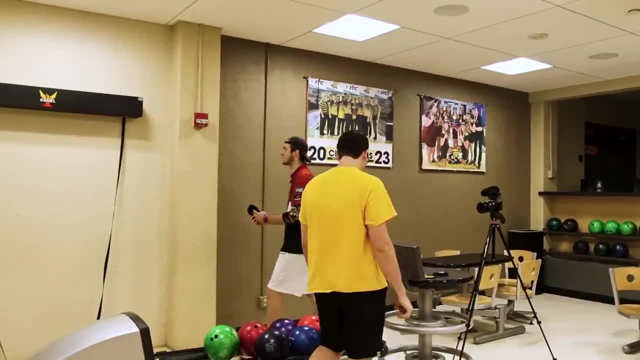 That's what I was looking at: Thump, thump, thump, thump, thump, thump thump. I think this is a strike Money Early lead. You got this one easy, Squeezing it at 200%. 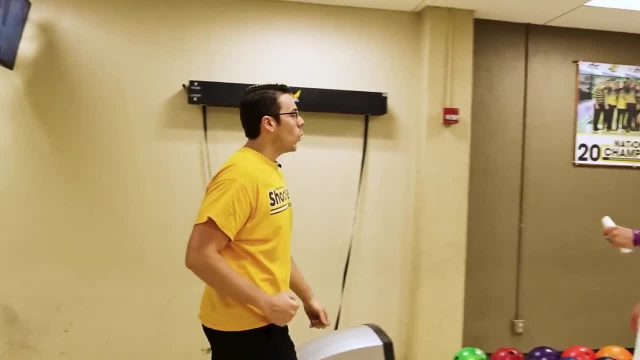 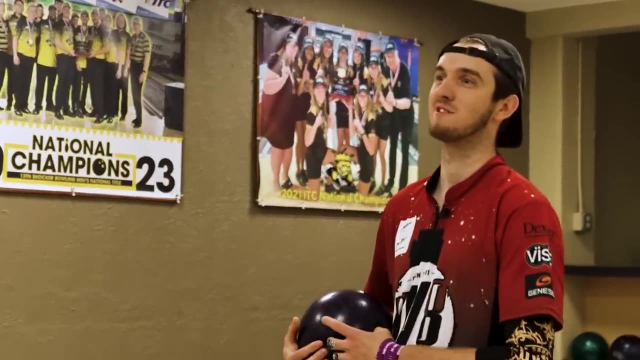 Oh, and you hooked it a little bit. Wow, Yeah, Yeah, I'm impressed. Oh, yeah, I'm impressed. That makes us what? two for six on single pin spares. now, Yeah, I'm still 0 for four. 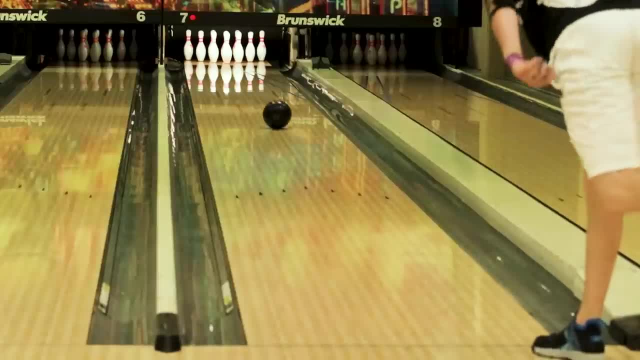 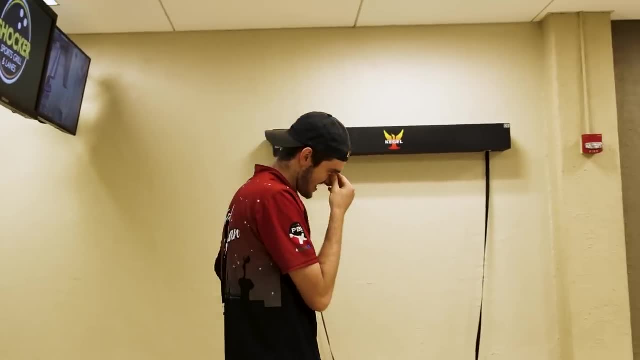 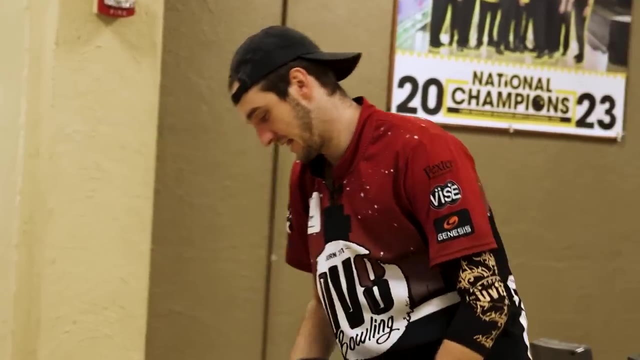 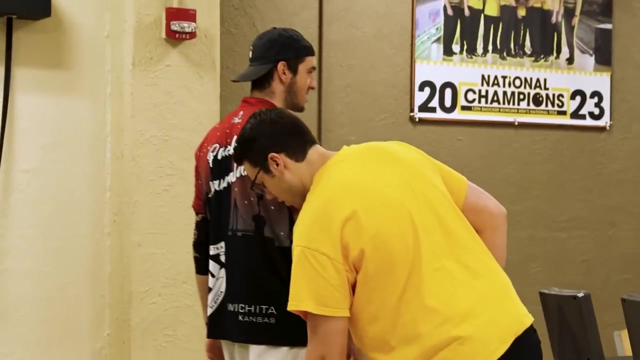 Oh, is that a double? Oh, That one hurt the soul, God. why did I say money when the ball was halfway down the lane? Money, Golly, Did he spare it? Nope, I got to change up the strategy. 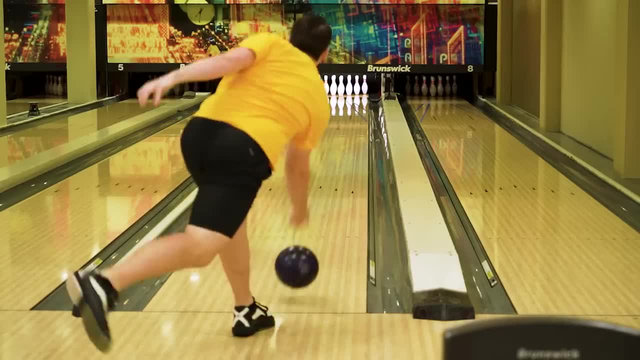 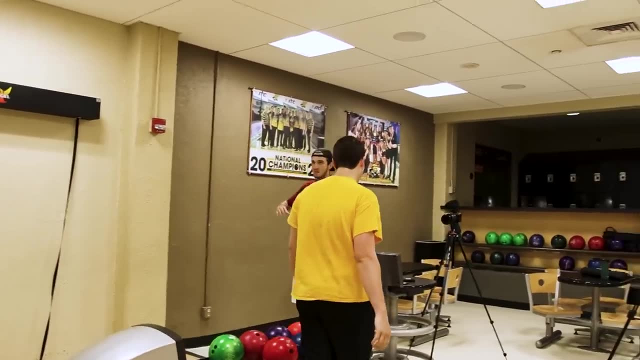 The whole going across the middle of the lane thing is just not for me. Ooh, Ow, Hoo, hoo, hoo. Come on, It's working. Until I can't fit my thumb in the ball, then we're going back to two fingers. 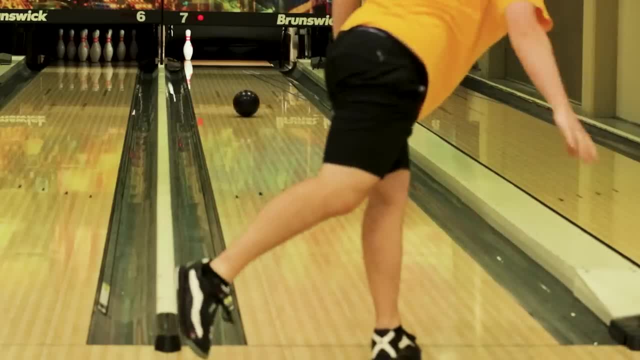 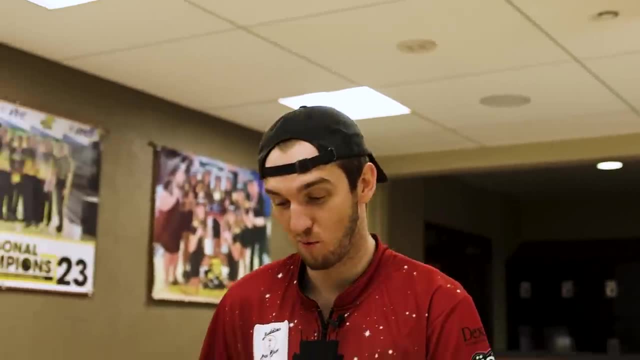 Then you're going to have to hook it a little. Yeah, Uh-oh, That was money the whole way. Yeah, I got to bank on the back half of this game him really messing up. Oh, Let me kick it here then. 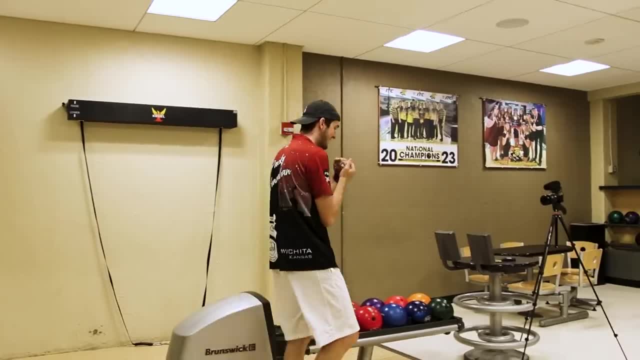 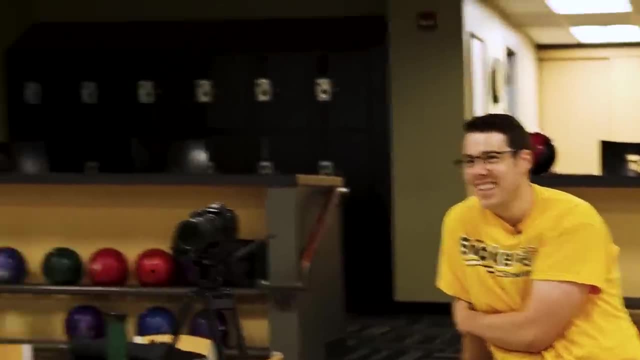 Ah-ha, I need to make my single pins. I need to make them. Looking at your conversion rate through the last seven frames, it's not very likely. It's 0% apparently. Oh, shooter, I can make spares two. 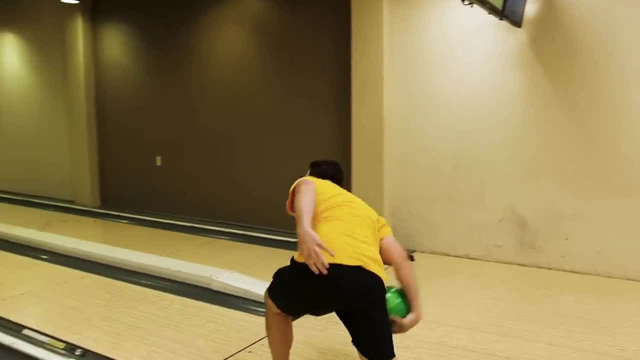 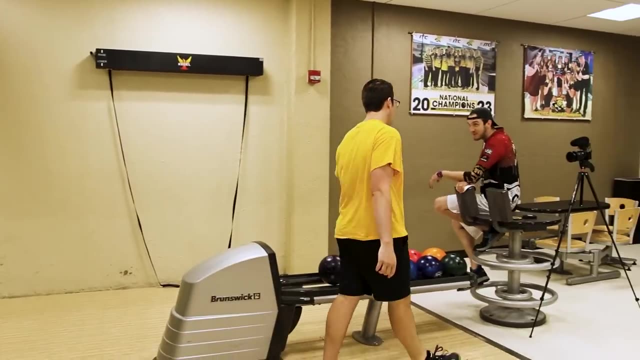 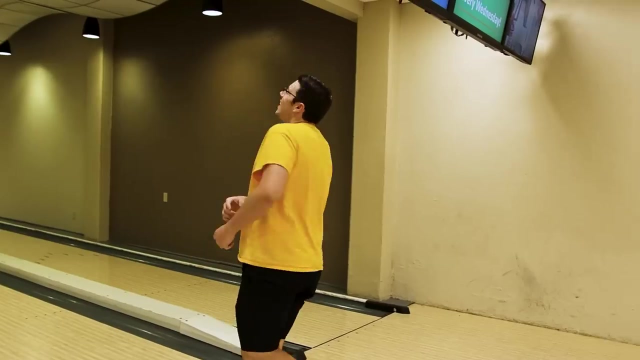 I can do it too. He's got to go back to hooking it, which has proven to be a challenge for both of us. Don't get on my ball, Come on. Don't put his thumb in. uh-oh, Uh-oh. 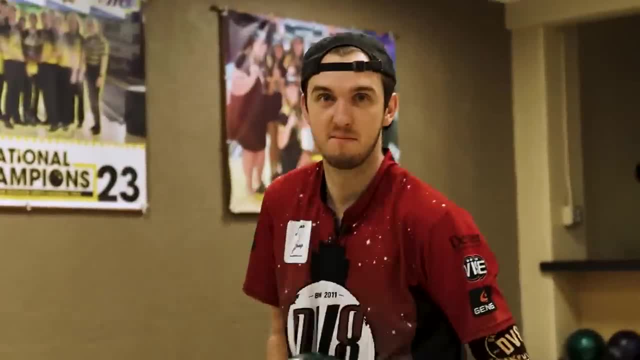 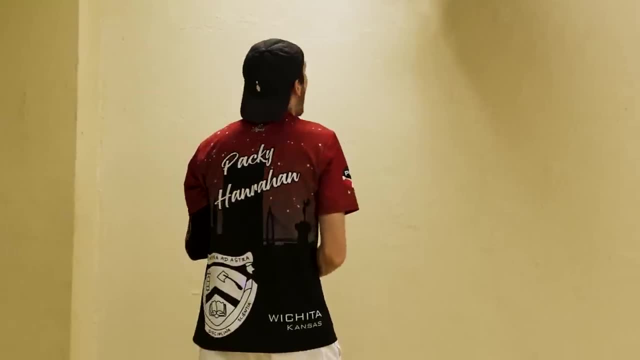 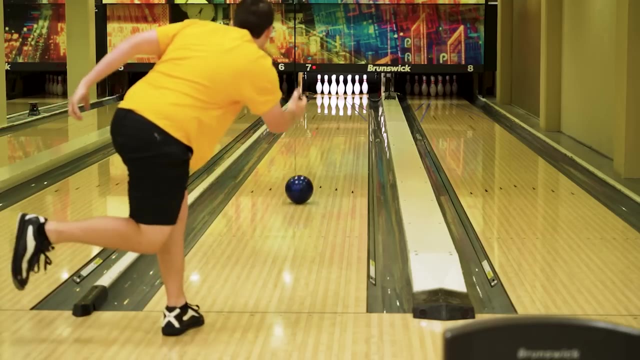 Great shot, Great shot. I'm back in the game. I'm back in the game. This is my time. Oh my God, my finger slipped out of the ball. My middle finger literally slipped out and went back in. Oh, that's Brooklyn. that's good. 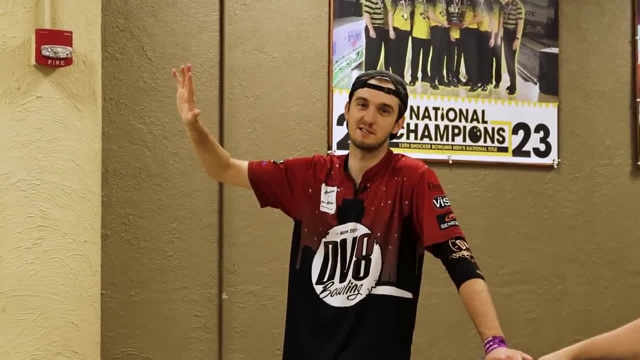 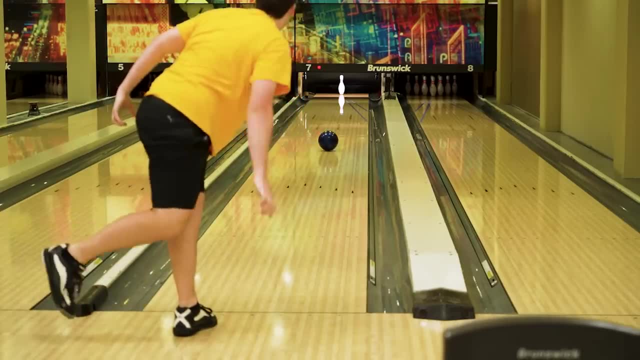 If you're watching on your cell phone, this is a time for you to put your hand up in the comments. My hand will be up in the comments. I don't know how they didn't strike. Please miss. Oh, I might have. 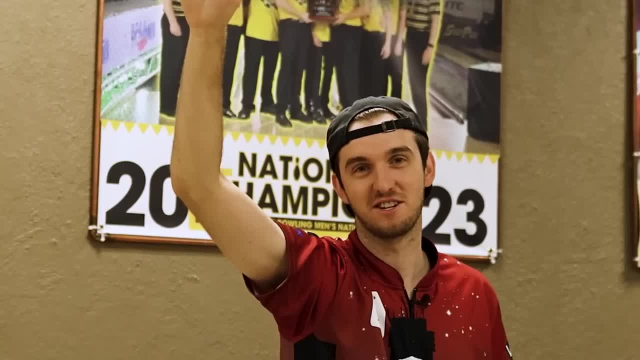 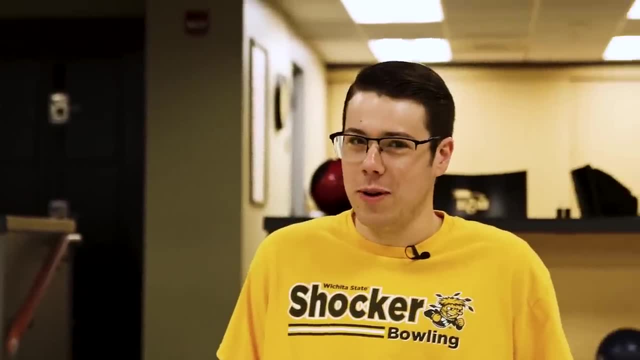 I want a chocolate milk. I'll take one large glass of element. Today's video sponsor. What a collapse the last two frames. let me tell you This is the worst barn burner you want to get into. Who can miss the most spares? 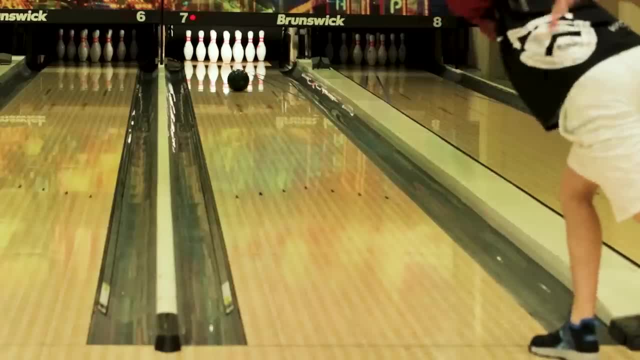 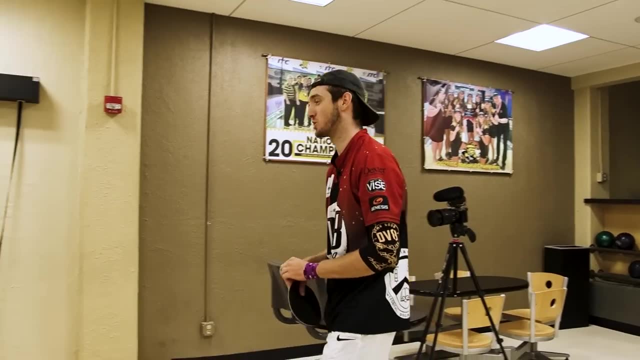 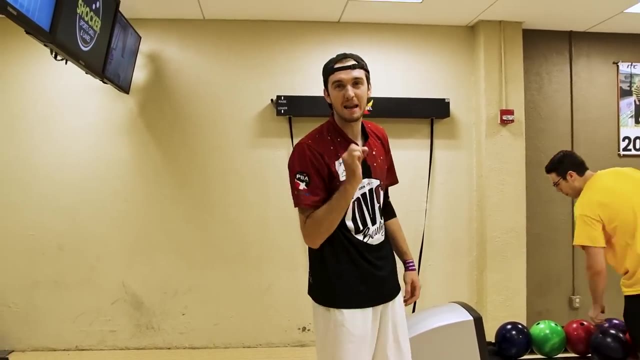 This is what it's come down to. I have money. Oh, stand up. nine pin Ooh, Come on dang. that was a good shot, Money. I figured it out. I told you guys and I'll say it again: 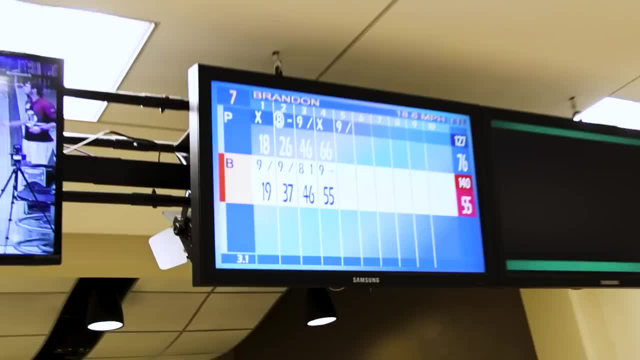 I'm not missing a spare for the rest of the day, For the rest of the match, not the rest of the day. I could beat you one handed. it's so easy. I'm kidding, I'm not saying that ever again. 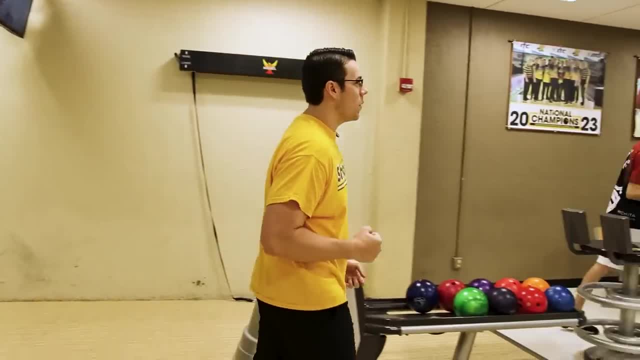 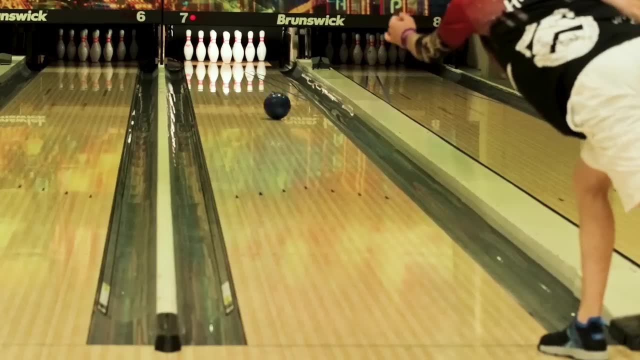 Yes, Oh boy, oh boy, oh boy, Come on. That's the last thing I need is a bunch of Brooklyns. Come on, Come on, 5-10.. Mmm, I feel like I finally found the groove and thrown it good. 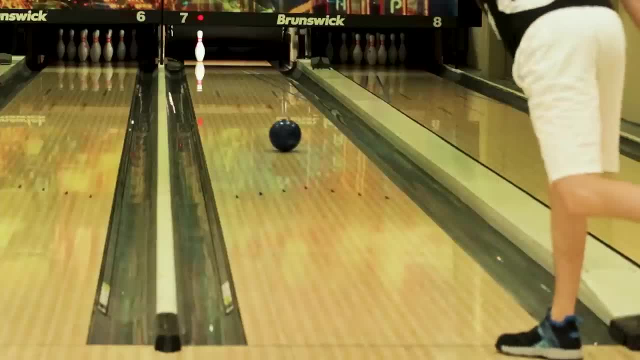 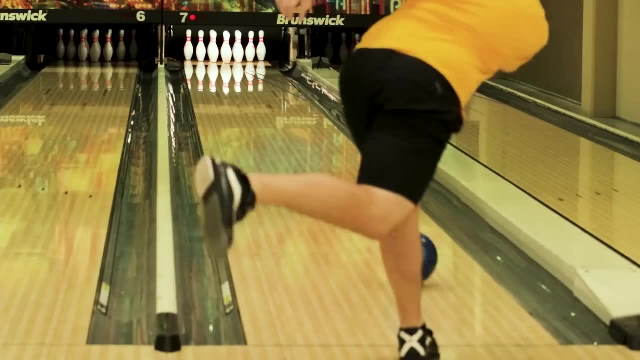 I went Brooklyn on purpose, just like I said. All right, Bears, This 1-2 pocket looks real nice right now. Oh, I hit the 3-2.. 1-2 pocket. I thought you hit the 6-7.. 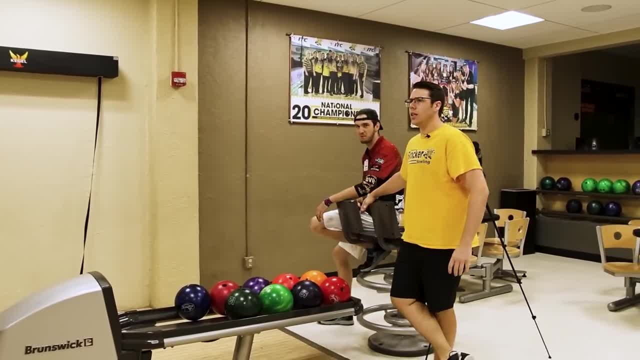 Yeah, that was the 4-7 pocket. Is that a 4-7?? That's a 4-7 pocket. Yeah, that is Over-rotated. the fingers on that one. That's a tough spare Good 2.. 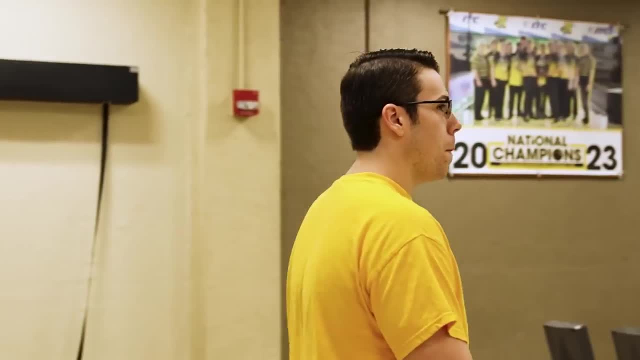 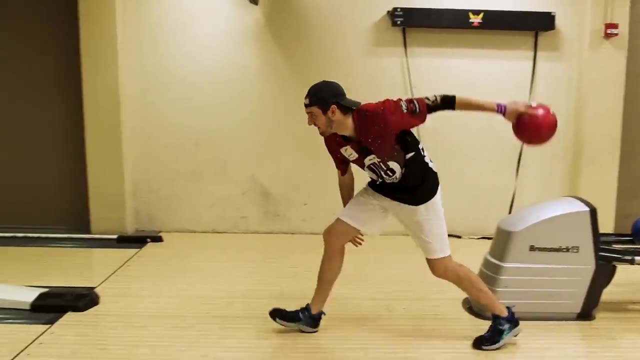 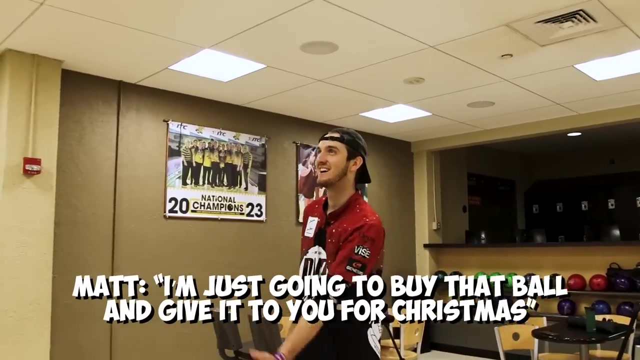 Good 2, though Good 2.. That puts me back in position. 10-pound ball. You know what that means. The rocket- Oh, All right, I'm going to buy that ball and just give it to you for Christmas. 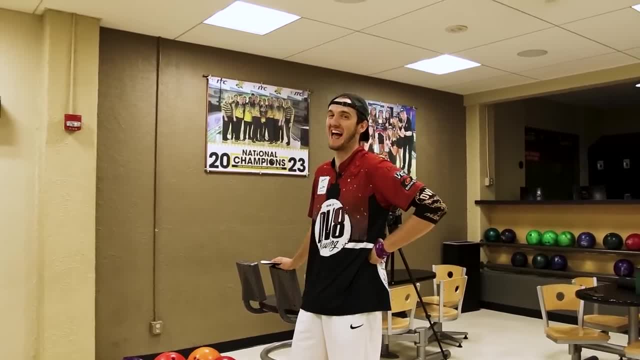 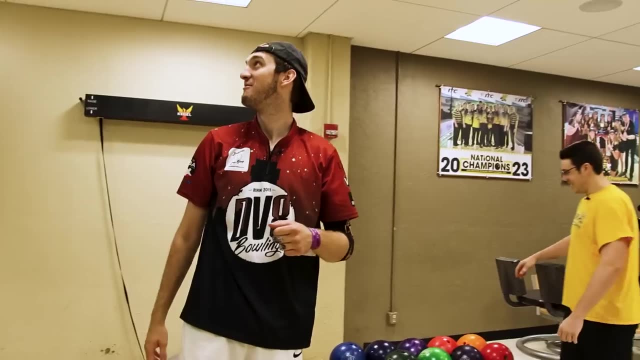 As long as you engrave my name on the top, I'm fine with that. Oh, he's locked. Four for four. Four for four. I am in trouble. We're looking like a 9th, 10th frame roll-off is going to be where we're headed. 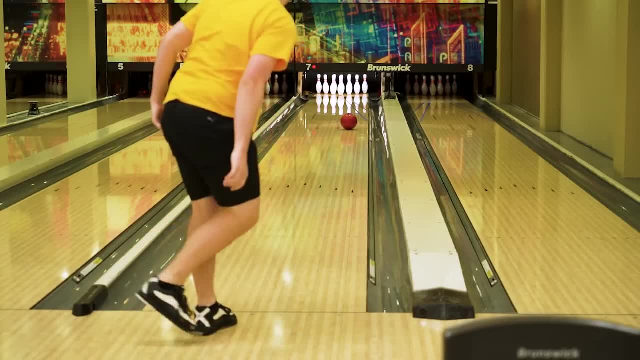 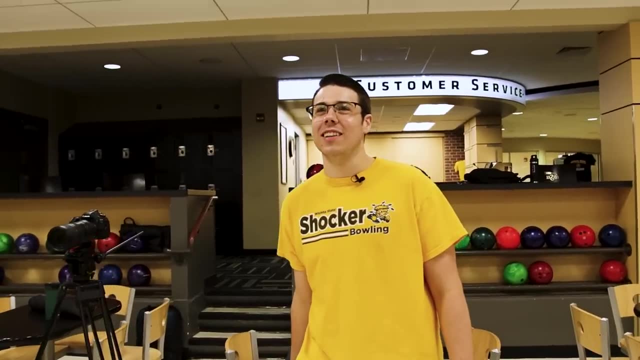 I'm going to have to throw some strikes. Oh wow, What the Come on. A little pink on the 10-10.. That's what we need right there. Maybe I just found myself a little groove. 9 pounds. 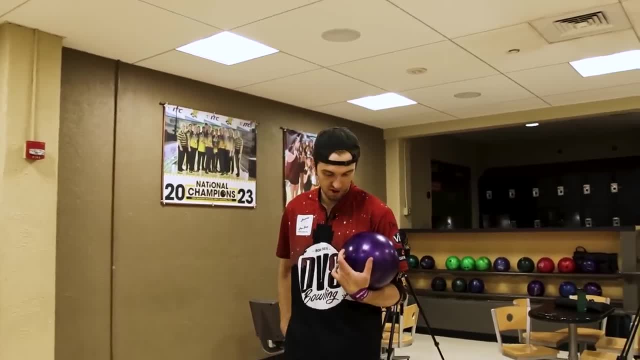 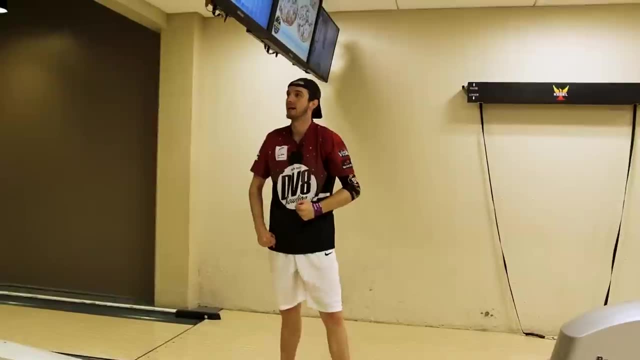 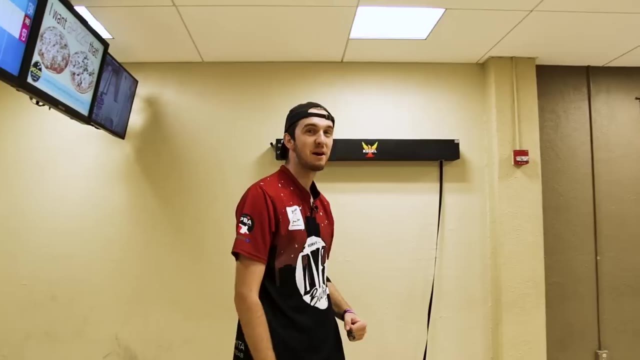 I'm really banking on the fact that this is a small finger hole and that'll be tough for Brandon to deal with. Oh my God, That was huge. The physics tell me I got to hit a little higher on the head pin to get a little less. 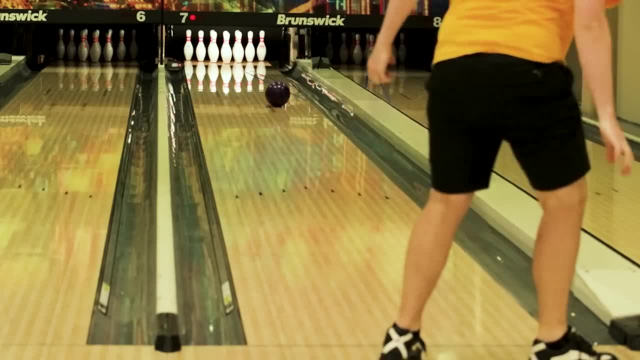 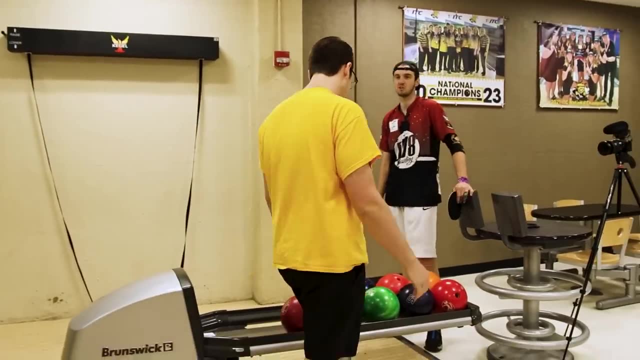 deflection. That's what I did, Uh-oh, Oh, no, Oh, not a 10-pin. Mine fell so yours could stand. You know what I'm saying: Unbelievable, That would have been a massive strike for you. 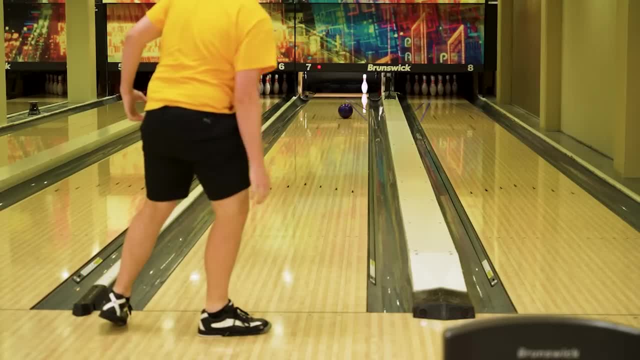 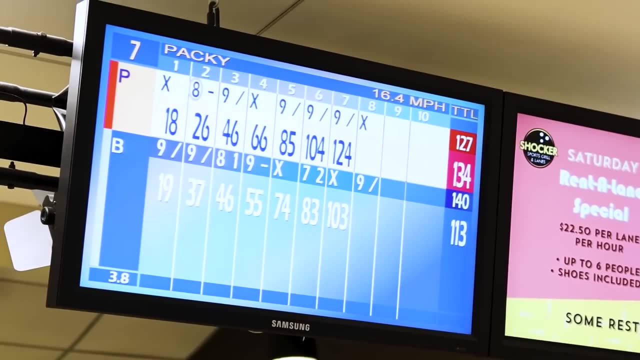 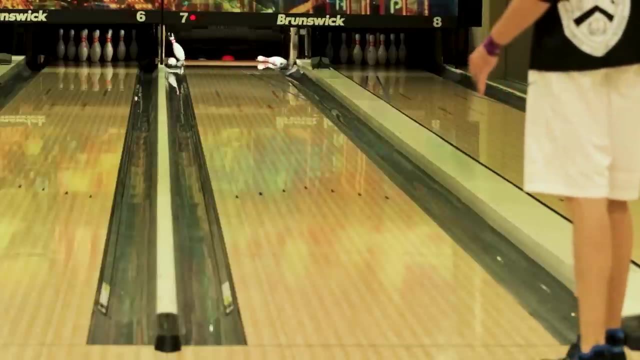 It would have been. It really stinks. Oh Woo, Skinny jeans, We've got the 8 and the 6 left. I just need you to do the right thing. Oh, that's pretty good. Oh no, That's good game. 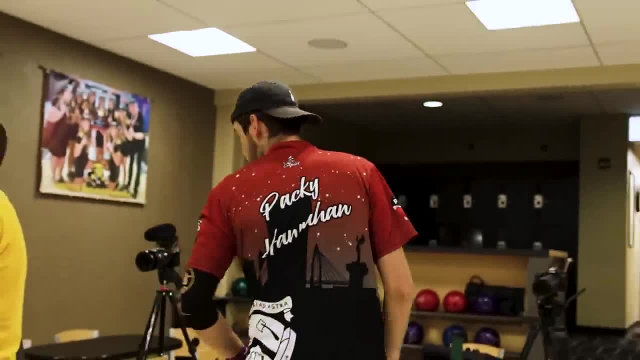 That's the ball game. That's the game. First double of the match. Was that really the first double of the match? That was the first double of the match. I mean spares for dough, strikes for show. It's a tough life when you can do both, you know. 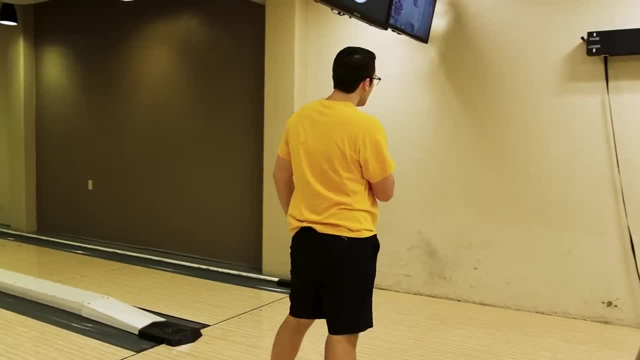 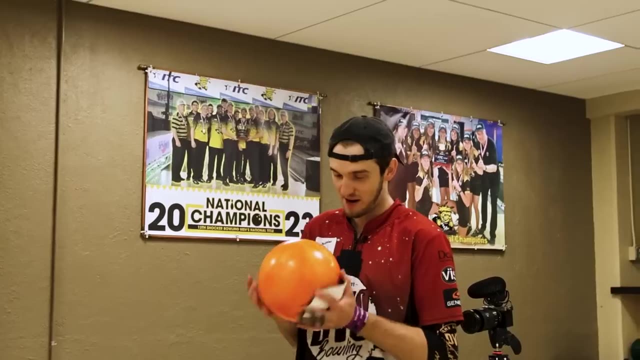 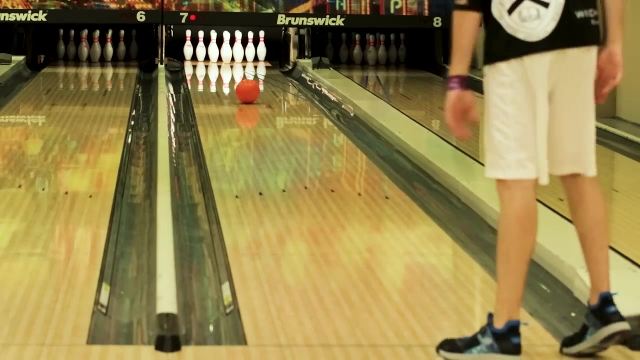 Oh yikes, That's tough. You did self-talk it right into getting two. Wow, We're going to use a 16 and a 6.. Yeah, this ball feels light. My guardian was tripled. The ball definitely went in front of the 7.. 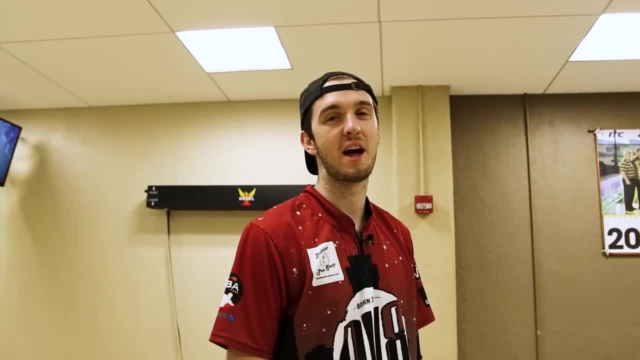 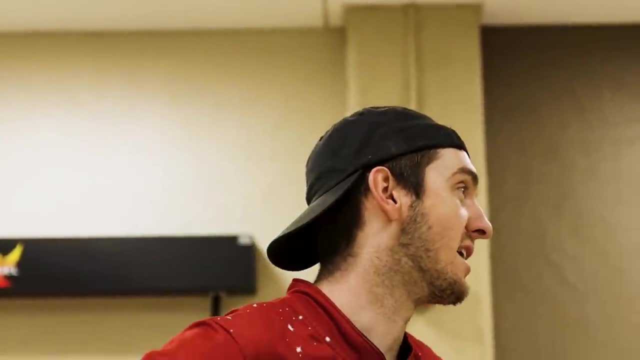 We have established ourselves a roll-off here. We have our 9th and 10th frame roll-off coming up, And there's one question that we have to ask Now. we've asked this to many people before: Brandon, do you want to go first or second? 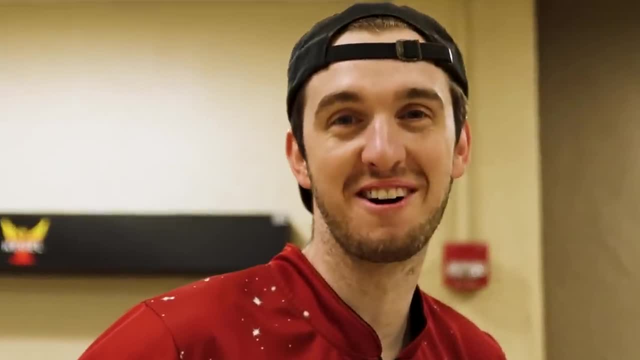 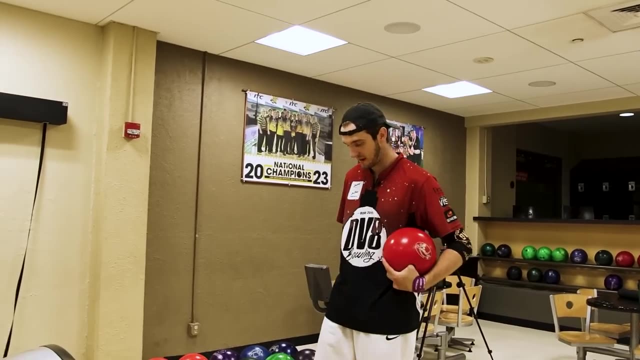 I want to go second. They always make me go first. 16-pound ball in the 9th frame. 6-pound ball in the 10th frame. I feel like I'm at the advantage with the 6-pounder, but at the same time, I feel like I'm at the advantage with the 6-pounder. 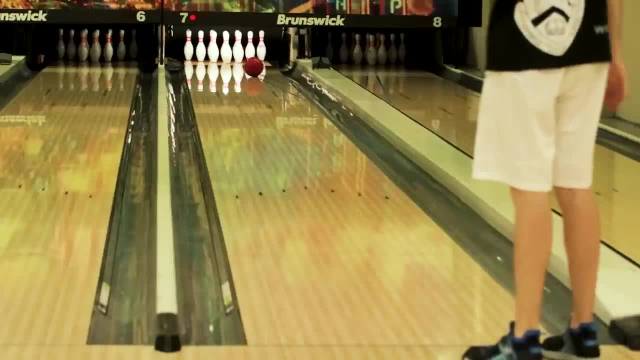 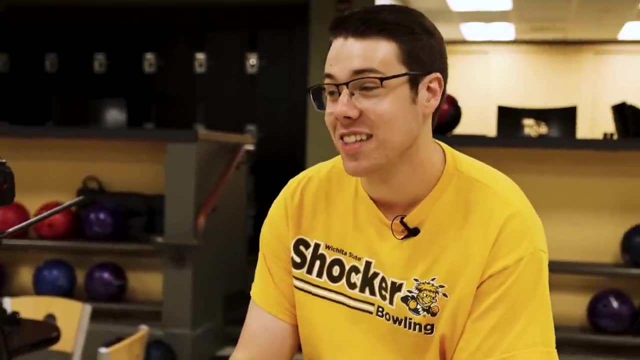 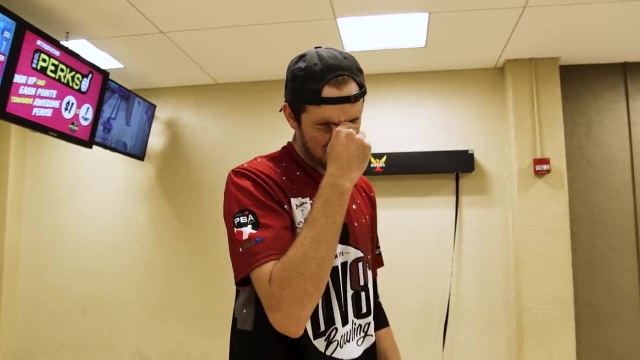 I feel like I'm at the disadvantage with the 16s. Oh, Stand up, 9-pin Stand. I was thinking that didn't fall. This is a make every time. Oh my God, Yikes, Yeah, it's just really hard to go from the 6-pounder straight to the 16..